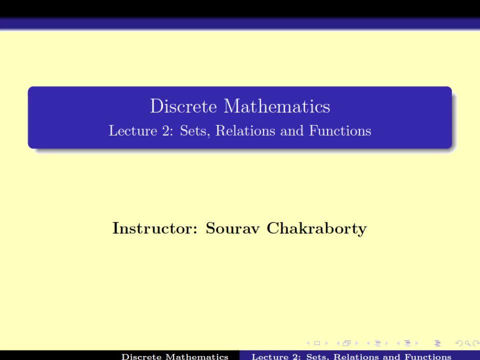 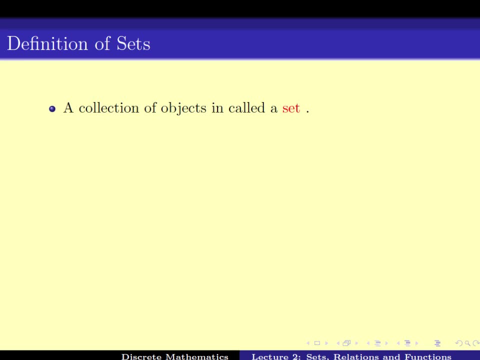 throughout the course. So it's very important for us to ensure that we understand these concepts very well. Let's start with the definition of sets. So what is a set? Any collection of object is called a set. The objects that comprises of the set are called the elements. 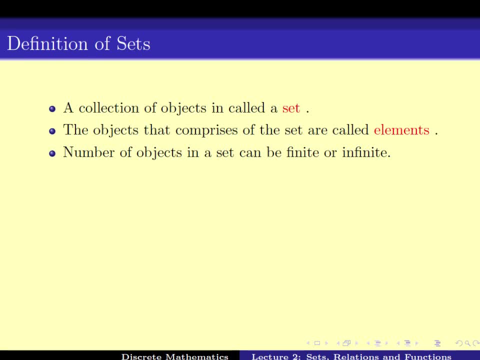 The number of objects in the set can be finite or infinite. For example, say, I can say a set of chairs, or the set of Nobel laureates in the world, or the set of integers, or the set of natural numbers less than 10.. So this comprises of 1,, 2,, 3,, 4,, 5,, 6,, 7,, 8,, 9. 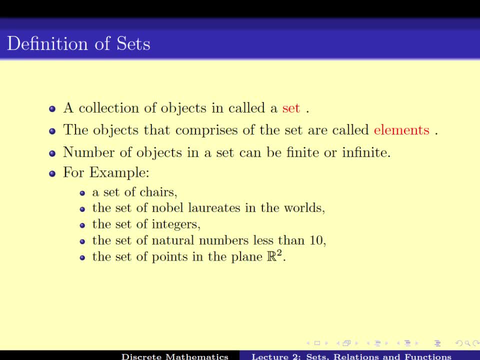 or the set of points in the plane r2.. Note that the set of integers and the set of points in the plane r2 are actually infinite. sets, Meaning the number of elements in the set are infinite. So we can have sets which are finite, or we can have sets which are infinite. 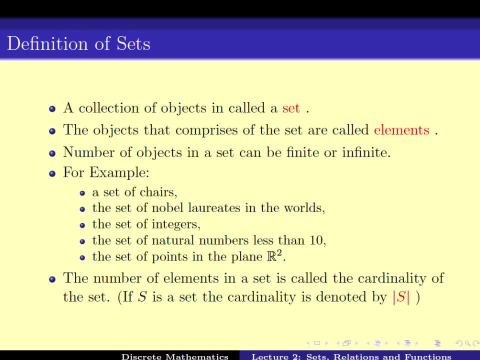 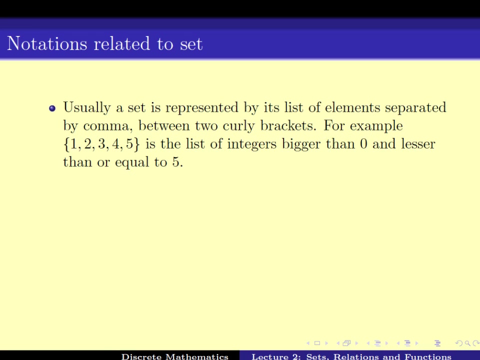 The number of elements in a set is called the cardinality of the set. It is usually denoted by this notation. So if S is the set, then S between two vertical lines denotes the cardinality of the set. Moving on to some more notations about set, Usually when I have to describe a set or represent a set, it 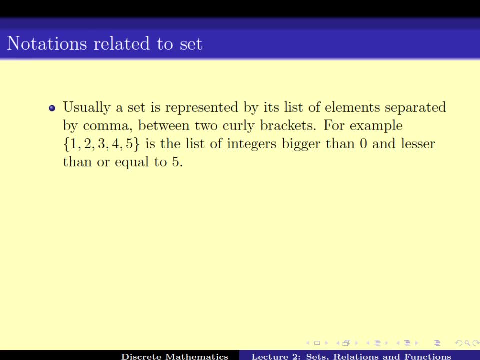 is done so by putting the elements separated by commas and between two curly brackets. For example, here, between these two curly brackets of this and this, I have the elements 1,, 2,, 3,, 4 and 5. They are all separated by the comma That. 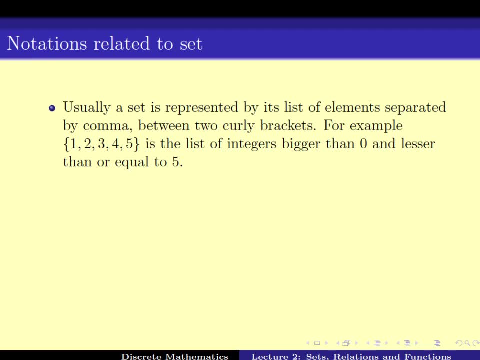 means this represents the set 1,, 2,, 3,, 4 and 5.. Now, if I have to pick an element out of a set, we usually use the notation of S contained in the set S. So this particular notation will be used again and again in 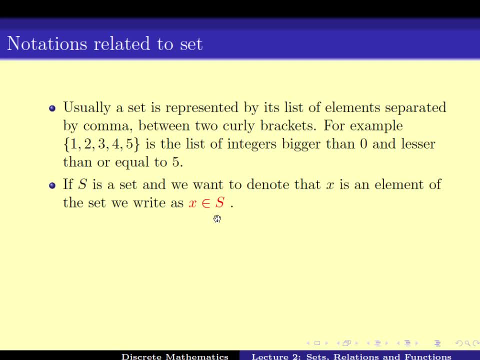 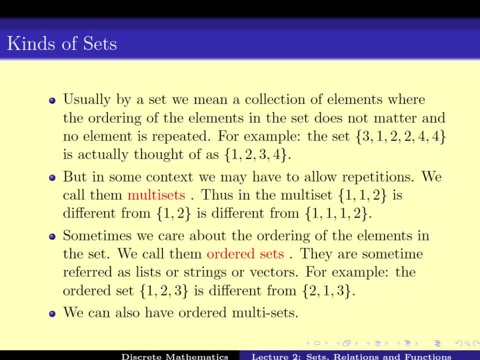 Now, if S is a set, I can take a subset of this S by taking some elements out of this set S. Now, if S is a set, I can take a subset of this S by taking some elements out of this set S. Now I have defined four different sets styles and this is very important for setting up the notational framework. 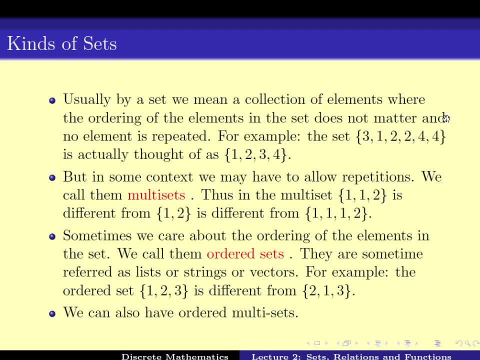 Firstly, when people talk about sets, they usually mean a collection of objects where repetition if not allowed and the ordering doesn't matter. So in this example, in the first example, If I tell you, the set comprises of the element 3, 1, 2, 2, 4 and 4, it is exactly. 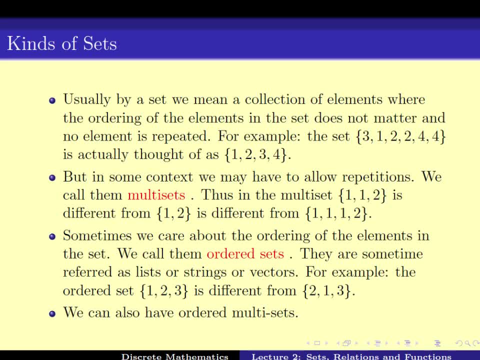 same as the set containing 1, 2, 3 and 4.. The repeated elements of 2 doesn't matter and similarly the ordering doesn't matter, But in certain context we might have to use these repetitions. These are called multi sets. 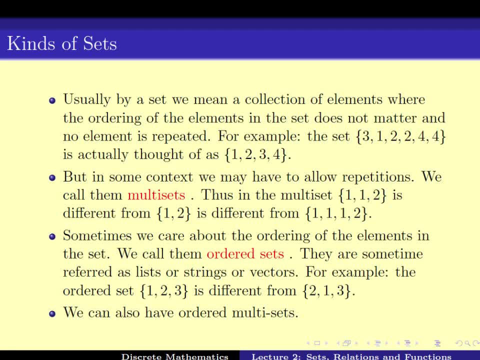 So Multi set is a set where repetitions matter. That means the set of 1,, 1 and 2 is different from the set of 1 and 2.. The reason being: in the first case- in set of 1,, 1 and 2, there are 2 1,s, whereas 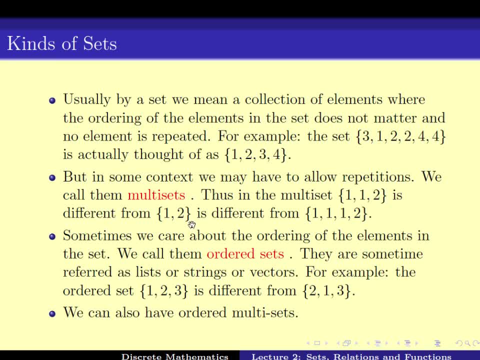 in the case one-two, there is only one-one, And similarly it is also different from three ones and two. So when we want to refer to such a set, where repetitions are allowed or repetitions should be taken into consideration, we call it a multi-set. 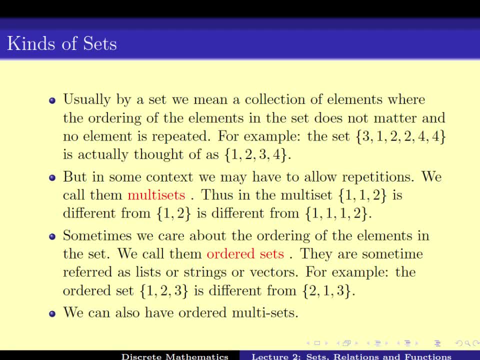 The third kind of set is what we call as ordered set. So these are the sets where the ordering matters. So that means that if I tell you the set comprises of one-two and three, this is different from if I tell you that the set comprises of three-two and one, or I say you that the 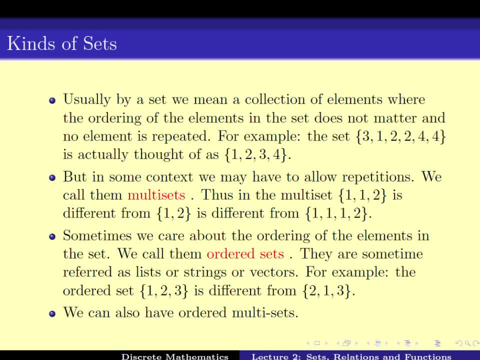 set comprises of three-one and two, Because the ordering of the elements in the set matters. So when we consider ordered sets, sometimes it has other names people use in different contexts. Sometimes it is called a list, A list meaning it's a list of objects or list of elements. 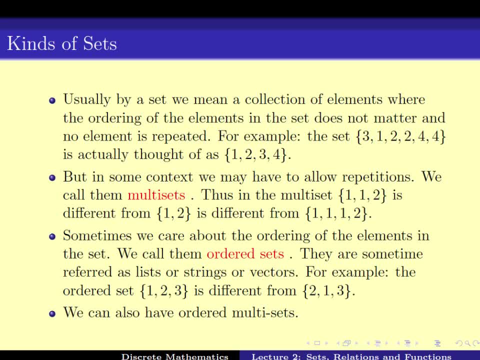 where the ordering does matter- See. similarly, we sometimes call it as string or vectors. Now we can also have sets which are ordered, multi-sets, Meaning sets where both repetitions as well as ordering matters. We will be using this terminology again and again in this course, So it is very important to get used. 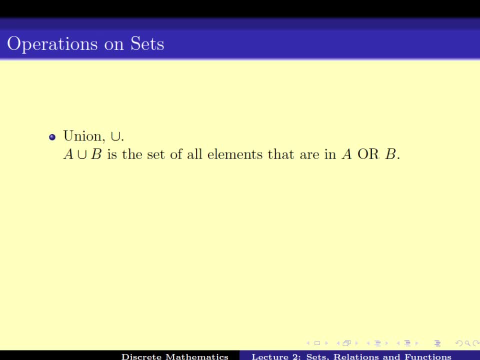 to this particular terminology. Now, given a set or given sets, we can have some set of operations on this set. There are three main operations that one can do, and they're pretty well known. First of all, is the Union So A-Union-B? 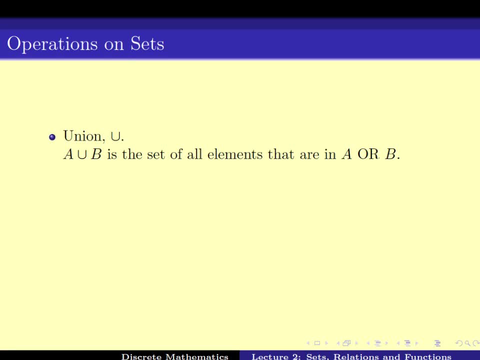 where A and B are two sets, is the set of all elements that is contained in either A or B, So it comprises of everything together. Similarly, there is the other one, which is the intersection. So A intersection B is the set of all elements that are contained. 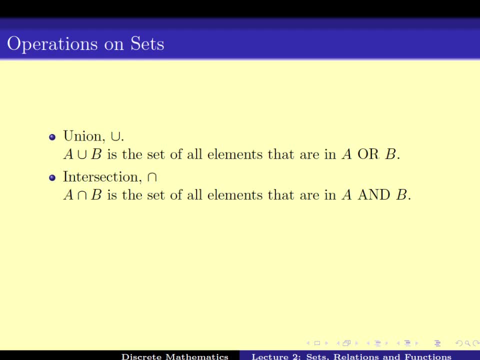 in both A and B. The third is the complement. This is the set of elements that are not contained in A. So this definition of complement assumes that there is a universal set- We sometimes refer it to U or omega- and the complement is the set of elements that are not contained. 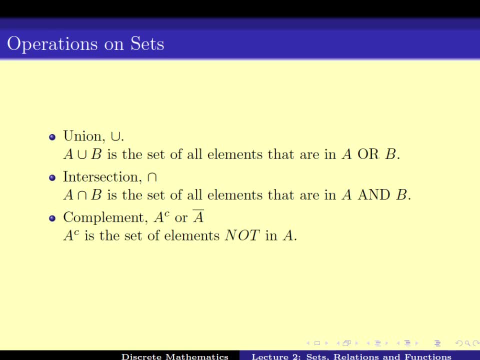 in A. The complement is all the elements in the universal set that are not contained in A. It is usually denoted as A power C or A with a straight line on top. There is one more operation on set that is done and that is called the Cartesian product. We will be. 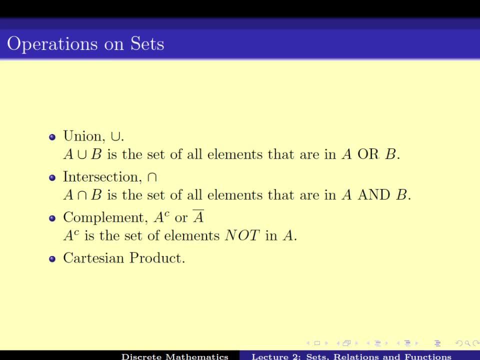 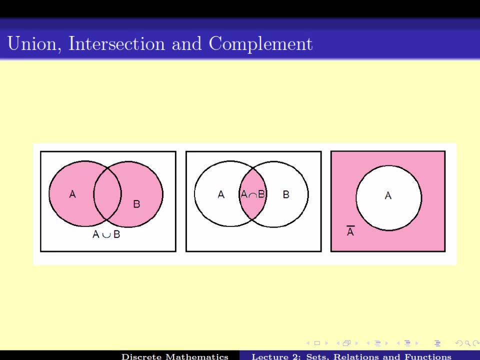 talking about this Cartesian product after a couple of minutes. So here is a pictorial description of union intersection and complement. So for example, look at the first picture. If A and B are these two round objects, so this round circle. 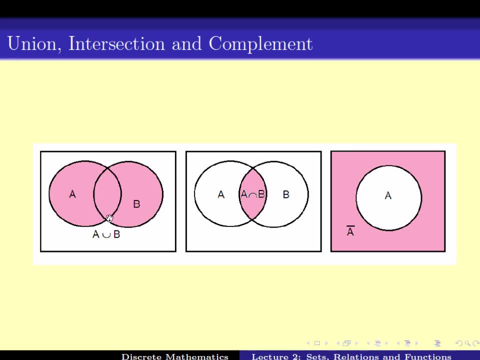 here represents the set B. Similarly, this round object here represents the set A and B. Similarly, the outer boundary wall, which is the rectangle, represents the universal set Same for all of them. Now, A union B is the set of all elements that are there. 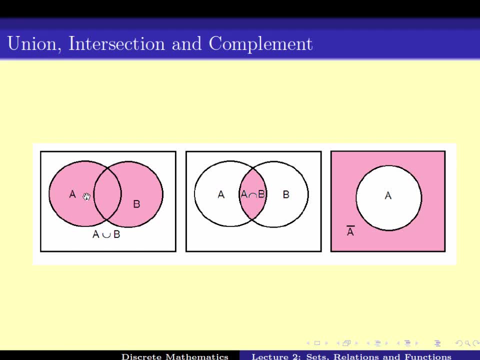 in either A or B or both. So it is all the elements that are there in the pink area in the first diagram. Similarly, A intersection B is the set of all elements that are in the pink area in the second picture and A complement is. 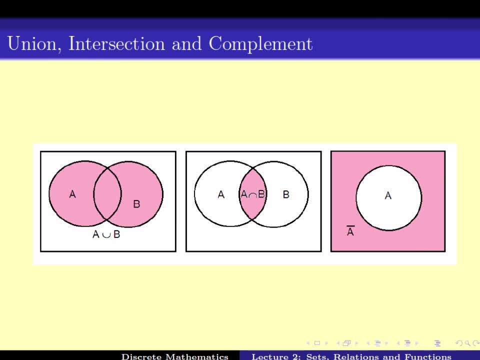 the pink area in the third picture. So this is what we call as Venn diagram, and we use this particular form of diagram a lot. Since it gives a pictorial view. it helps us to think in a slightly more easier way. Now the set of these three. 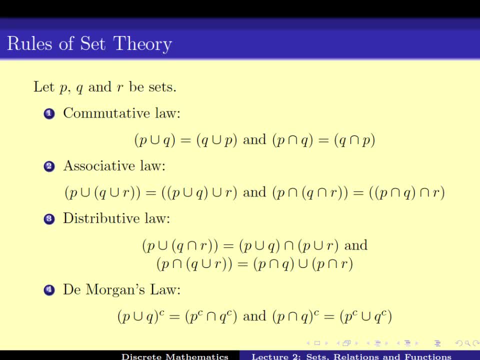 operations that are there, that is, the union intersection and complement satisfies some set of laws. I have written down some obvious set of laws. these are the most natural ones and most important ones. Number one is this commutative law, which means that P union Q is same as Q union P and P intersection Q is same as Q intersection P. 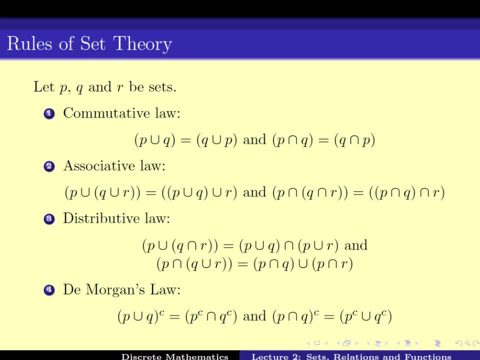 The other law is associative law, which says that P union, Q union, R is same as you first do the union of Q, P and Q and then you do a union with R, Similarly for the set of intersection. This is called the associative law. The third law, which is an interesting law, is the distributive. 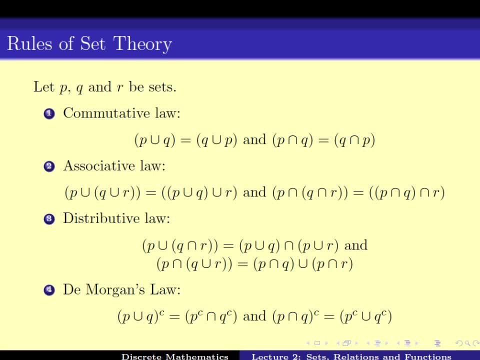 law. This tells that P union Q intersection R is same as you first do the union of P with Q and P with R and then intersection with it between these two sets. Similarly, P intersection Q union R is same as P intersection Q un Democracy. 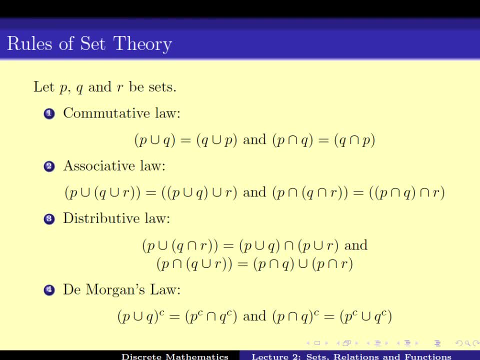 turns out intersection are. And the fourth law is the De Morgan's law, which says that P union Q complement is same as P complement, intersection Q complement and similarly, P intersection Q complement is P complement, union Q complement. Now these laws are provable laws. That means you can prove these laws from the 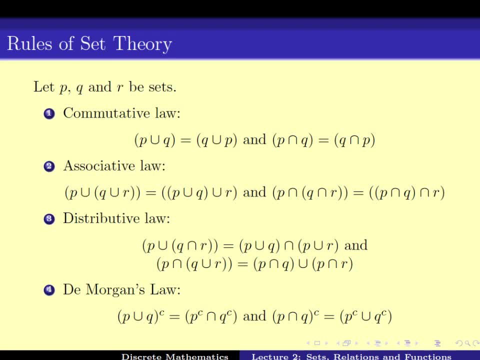 definition of intersection and union and complement. I leave it to you guys to check that these laws are indeed correct. In the two video lectures that I will spend on solving problems, I will prove that these laws are actually true, Thank you, But before that I encourage you guys to prove it for yourself, or try to prove it. 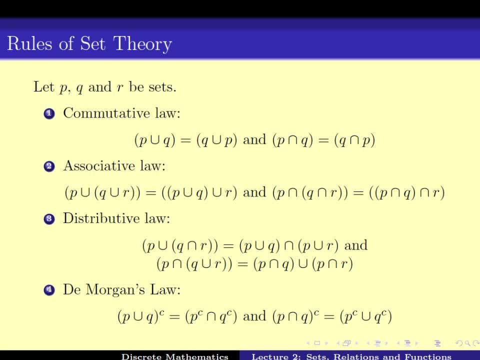 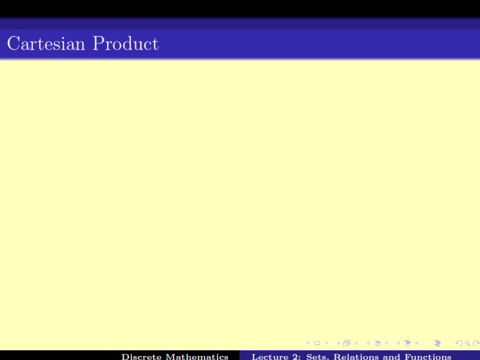 for yourself that these laws are indeed correct. They should follow from the definition of union intersection and complement. Now, as I told you, there is one more law other than union intersection and complement, and that is called the De Morgan's law. In the preached we can say that when a Eggs and Cubes are mentioned by process, 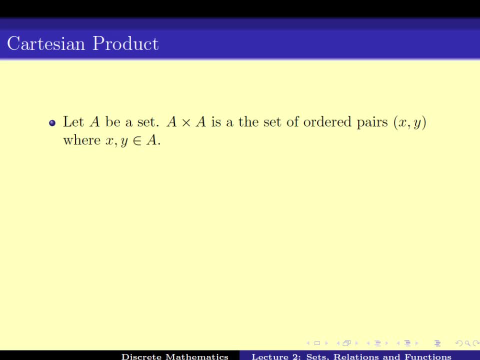 let's say there's one product and we want to change the process of acting upon it. let's say this is escrever the new colleague. Let's put the order column of that Zielce. it's a literal error capable of increasing the number of. 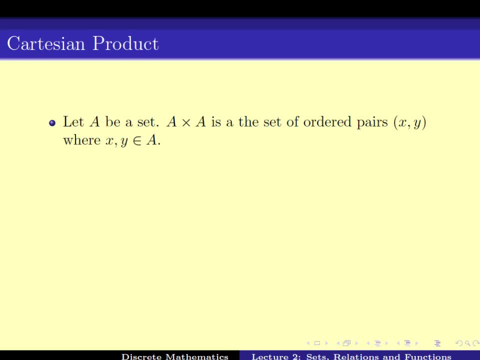 provides level to smaller cases, because did you know that, protected surrounding by the 죠第-'CZ'而已 and critical data library, 엄청 important detective. nous l'analyze un être iligers, il 밖에 n'est dit quitte. 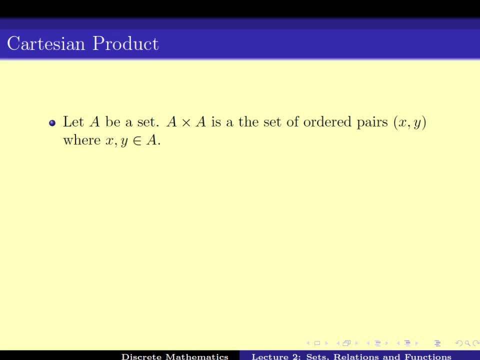 dans une é Fanidieria. Delphine carte. initial regarding over by the operation on sets y, the ordering of x and y matters, So x, y is different from y, x. Here I have given you the definition of A Cartesian A. You can also do the definition of A Cartesian. 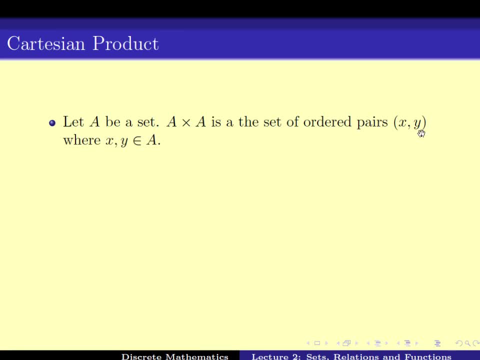 product B, where it is the ordered pair x and y, where x is in the first element, first set A, and y is in the second set B. So similarly you can define the Cartesian product between any two sets A and B. When you have to do something like take the Cartesian product. 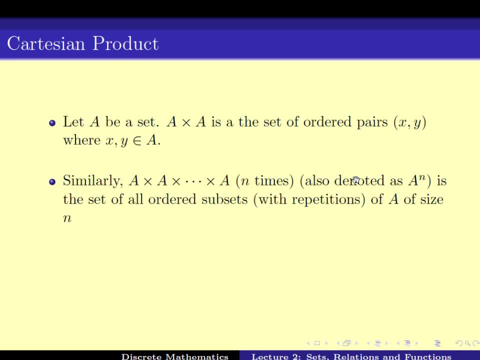 of A a number of times, say n times. we sometimes denote it as A power n. So in other words, in the above example, a Cartesian a can be written as a square. Similarly, if I take the Cartesian product of a n times, I get a power a. 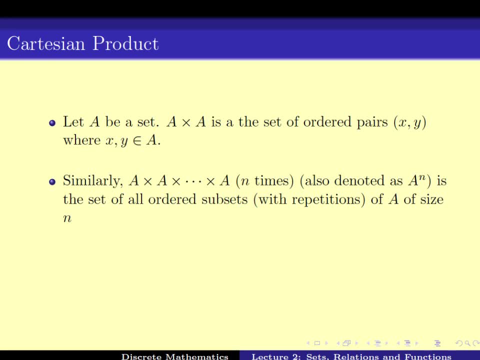 And what is this? If you unfold the definitions of Cartesian product of a with a, you realize these are the strings of elements of a of length n. In other words, these are the ordered subsets with repetition of a of size n. For example, if a is the set 0, 1, then 0, 1 power n is the string of 0 and 1 of length. 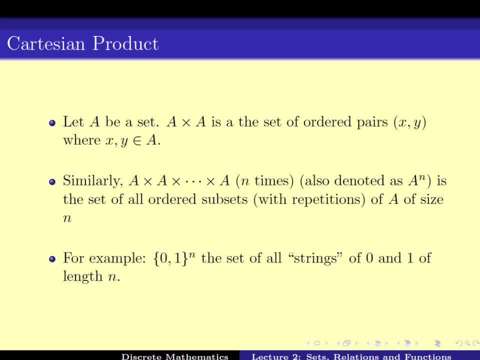 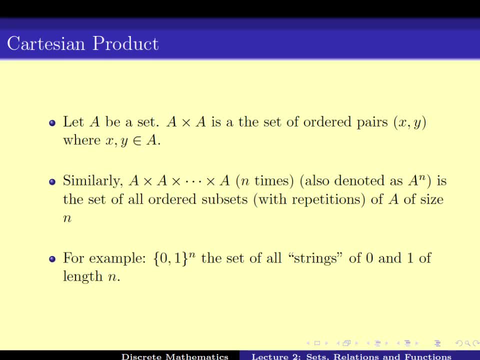 Similarly, 0, 1 power. 3, 0, 1 cube is the set comprising of the strings 0, 0, 0, 0, 0, 1, 0, 1, 0, 0, 1, 1, 1, 0, 0, 1, 0, 1, 1, 1, 1, 0 and 1, 1, 1.. 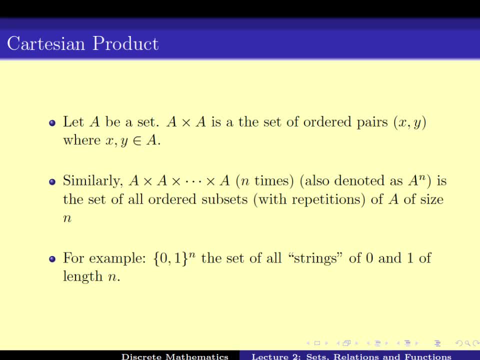 So it is all the strings of length 3 comprising of 0 and 1.. Now this particular object of 0 common 1 whole power n is particularly interesting for us, Since in computer science we do work on boolean things all the time. that means we are only 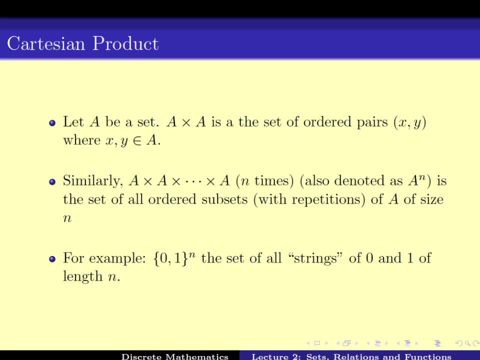 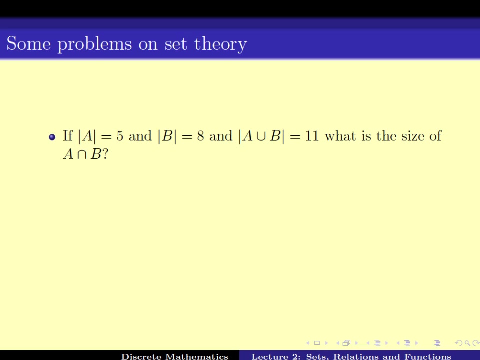 interested in 0.. 0 and 1.. 0s and 1s, So 0,1 appears again and again. So this set of 0,1 power n is called the hypercube or the n-dimensional hypercube. Now let me end this introduction to set theory by giving. 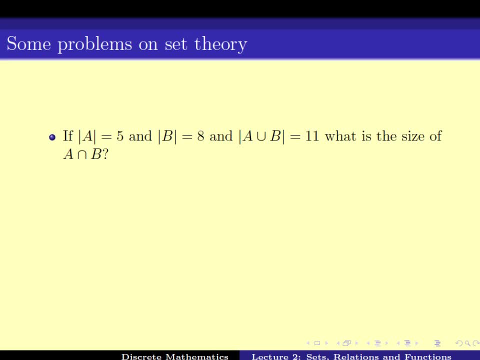 you some problems on set theory. I will be requesting you guys to do this problem as a homework for your better understanding of this subject. I will use the video lectures that I dedicate for problem solving to give you solutions to these problems. So here is the three problems that I have listed out for you. You can take down and. 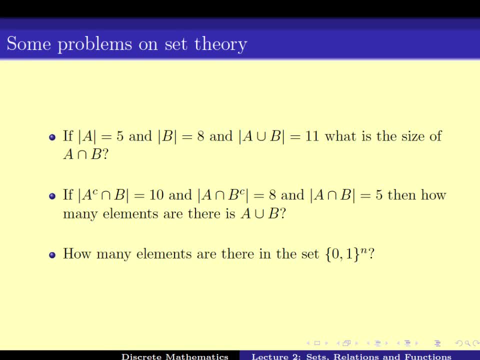 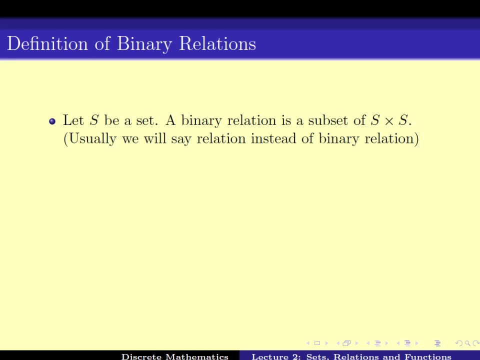 solve them. Now, moving on, let's move to the next important abstract object. This is called relation. In particular, we will be looking at binary relation. So what is a binary relation? So, if s is a set, a binary relation is a subset of s cross, s or s Cartesian product with s? 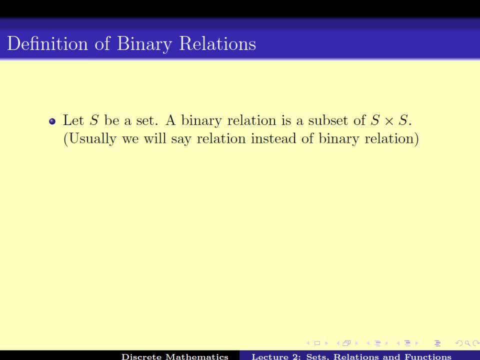 We usually call this one relation, so more correctly it should always be called binary relation. So if R is a relation on the set S, that means R is a subset of S, Cartesian product, S, and if this ordered pair of X, Y is in this R, we say X is related to Y. Sometimes we 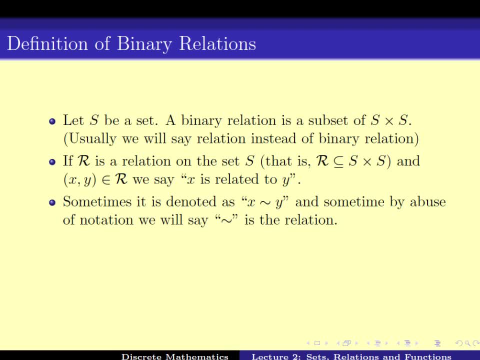 denote the relation with this kind of a tilde notation, and this is used as saying that X is related to Y. Binary relation is an outstandingly powerful tool to represent various complicated situations, and it is heavily used for modeling of real life problems and mathematical problems. 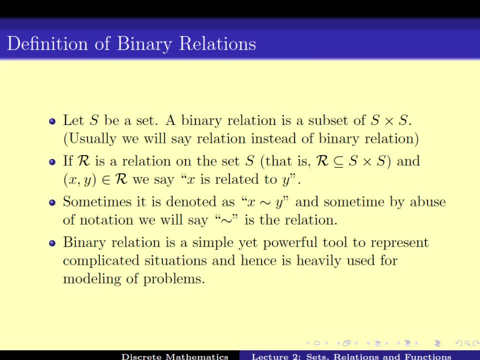 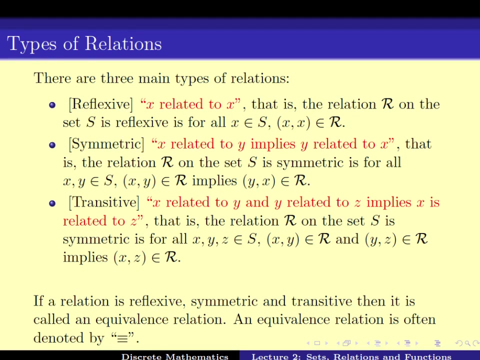 We will see how this binary relation can be used for modeling problems in the due course of this video lectures. In fact, understanding binary relations is one of the central subject in whole of mathematics and computer science. The binary relations, depending on whether they have some more structure or not, has been 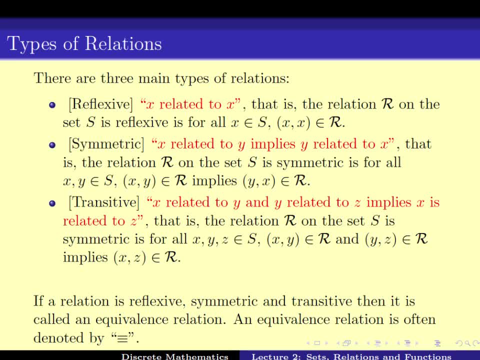 classified into various categories. So here are three main types of binary relations. Number one, what we call as reflexive binary relation. so in other words, X is related to X, So X, comma, X is in the binary relation R. Second one is the symmetric binary relation. 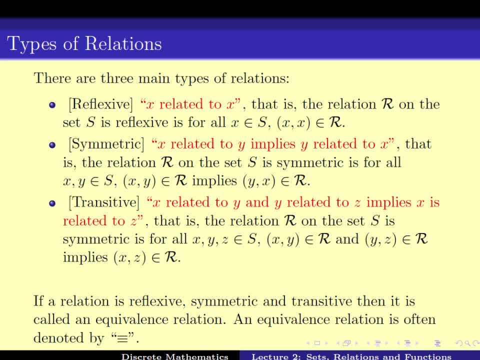 so here, if X is related to Y, that means Y must be related to X, or in other words, X comma Y is in R If, and only if, Y comma X is in R. The third is the transitive relation, where if X comma. 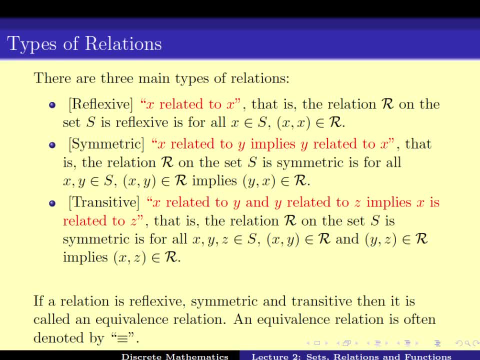 Y is in R and Y comma Z is in R, then it implies that X comma Z is also in R. So if X is related to Y and Y is related to Z, then X is also related to Z. So these are the three main types of relation, depending on the structure of the binary relation. 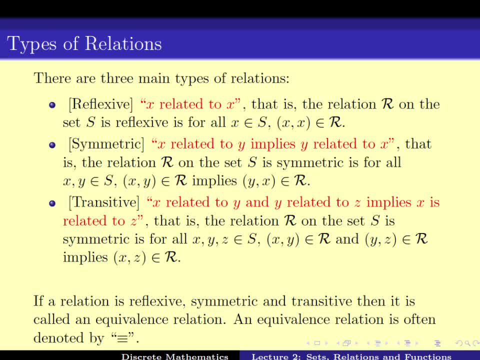 or the subset of S, cross S. that defines the binary relation. If a binary relation has all the three properties, that is, it is reflexive, symmetric and transitive, we call it an equivalence relation, Equivalence relation, Equivalence relation. 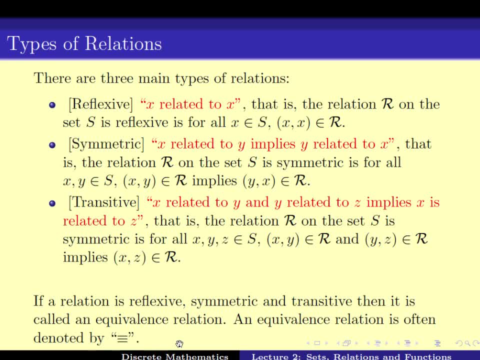 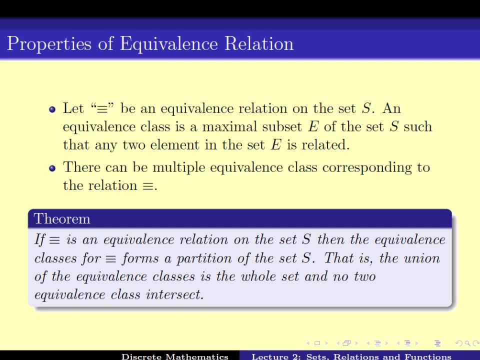 Equivalence relations are usually denoted by this particular sign of three horizontal lines. Now let us consider an equivalence relation. Now, given an equivalence relation, I can define a maximal subset E of the set S, which of the set S, such that any two elements of the set E is related to each other. 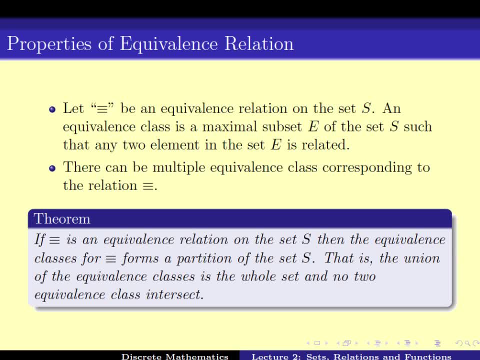 It's maximal in the sense that you cannot add any more elements to the set E by still maintaining the property that any two elements in E are related. It's maximal. it cannot be grown any further. So once I get such a set E, I call that E an equivalence class. 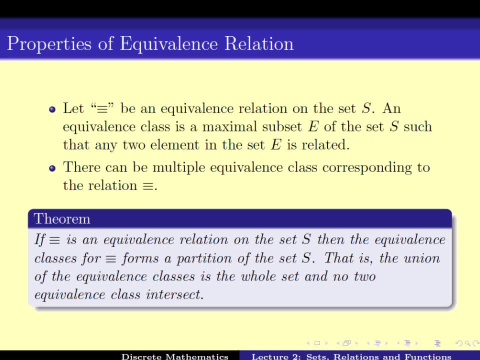 Given an equivalence relation, there can be multiple equivalence classes, or in other words, there can be more than one set such that there can be multiple equivalence classes. Any of those sets are maximal and any two elements of those in any of the set is related. 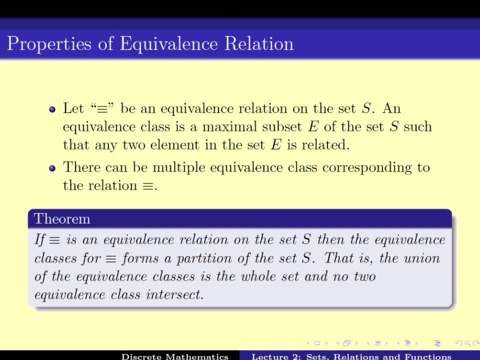 Here there is a beautiful theorem. It says that the set of equivalence classes partitions the set S. That means the union of the equivalence classes gives you the set S And no two equivalence classes can intersect. This is a theorem. This theorem again follows from the definitions of equivalence relation and equivalence classes. 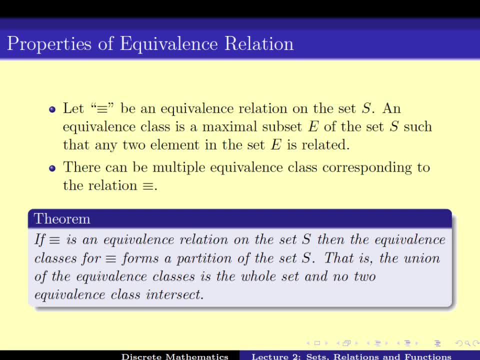 It is not an hard theorem to prove but, like many other theorems, the implication of it is pretty enormous. Again, I leave it as an exercise for you to try. I will give a proof of this theorem in the video lectures where I will do the problem. 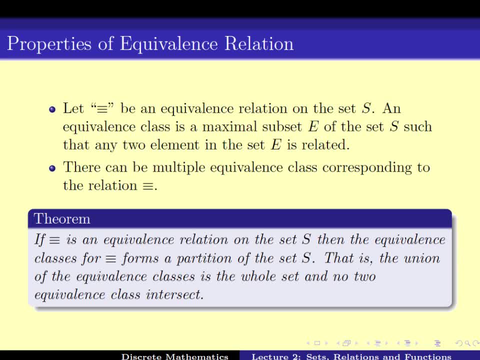 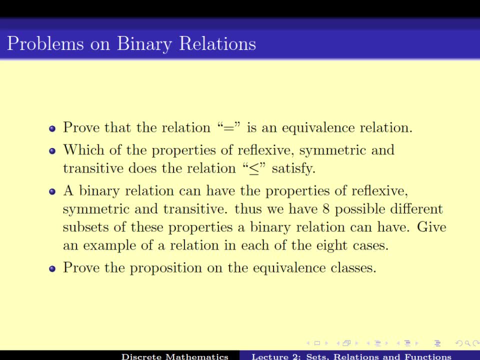 sets. I will be giving you the formal proof of this theorem. Till that time, I request you guys to try to solve it for yourselves. Here is a list of problems on binary relations that you should attempt to solve by yourself. They are all easy and should follow from the definition of binary relations. 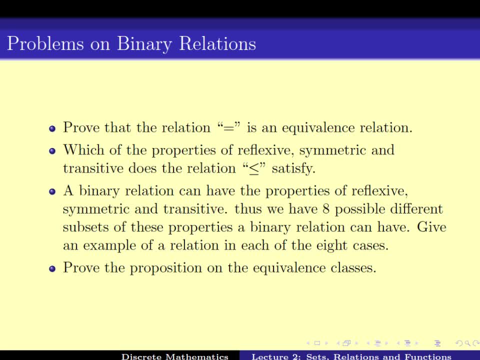 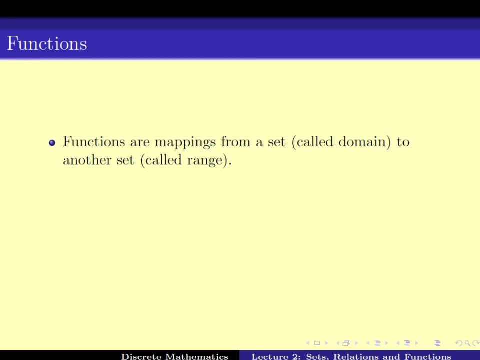 Moving on, let us tackle the third important concept, or abstract concept, and these are called functions. So what are functions? Functions are mappings from a set which we call a domain to another set which we call range. So it is very simple. 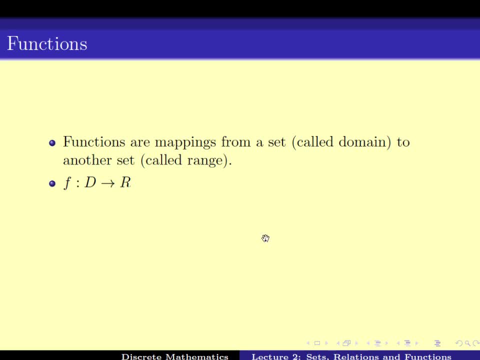 It is very simple. It is very simple So it is denoted like this: So f from a domain D to a range R. The function has some nice properties that for every element in the domain X, the f of X or the mapping of X is well defined and must be in the range. 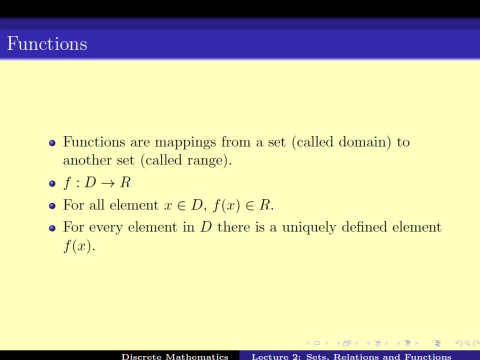 R, Again another property. For every element in D there is a uniquely defined element f of X. That means you cannot have X mapped to two different elements in the set R. If a mapping satisfies these two properties, we call that a function. 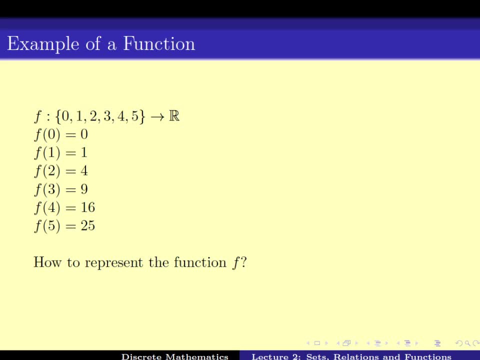 For example here. take this function. This is a function mapping from the set 0,, 1,, 2,, 3,, 4 and 5 to the set of real numbers. For example, f of 0 is 0, f of 1 is 1, f of 2 is 4,, f of 3 is 9, f of 4 is 16 and f of 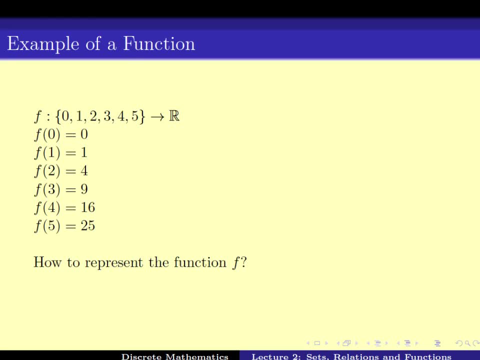 5 is 25.. You can check that f of any element of the domain is well defined and unique and hence it is a function. So what is a function? Now? how do you represent this function? Note that I have given you this function explicitly. 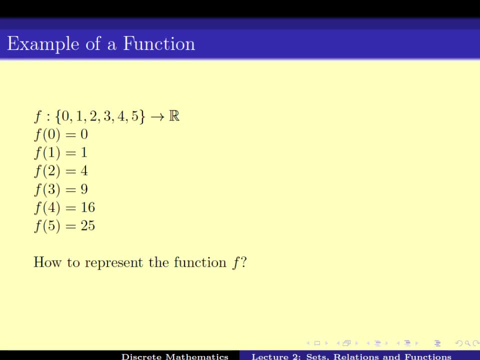 That means, for every element X in the domain set, I have specified what is f of X. Thus you can represent a function explicitly by giving the function, or you can come up with some pretty clever way of doing it. So what is a function? 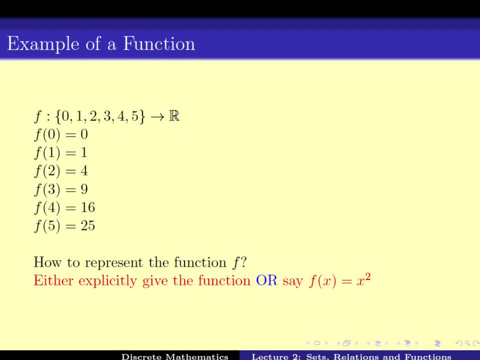 There are several ways of defining it. For example- here you can check that I could have just told f of X is X square. So you can either explicitly give the function or implicitly give a nice equation for the function. When somebody gives you the function explicitly, we call it a truth table. 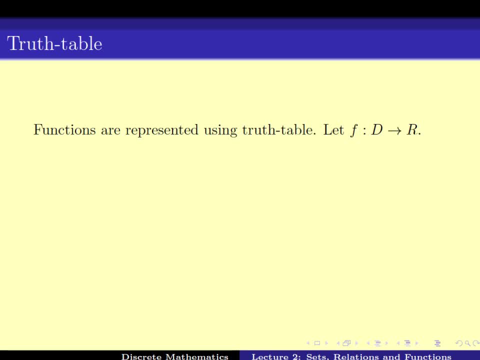 The functions are represented using truth tables. So how do I represent the function using truth tables? So, for example, if I have to describe a function to you, one way is that we mutually agree a ordering of the domains, The domain set. so let us say that: okay, see, the ordering of the domain set is X1,. 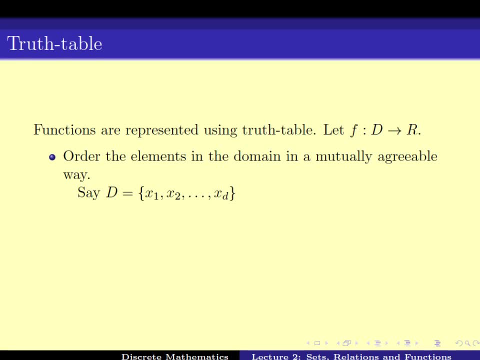 X2, X3, dot, dot, dot till Xd. Okay, Now, once that ordering has been pre-determined, I can just give you f of X1,, f of X2,, f of X3, dot, dot, dot, f of Xd, and you will immediately understand that when I the third element, 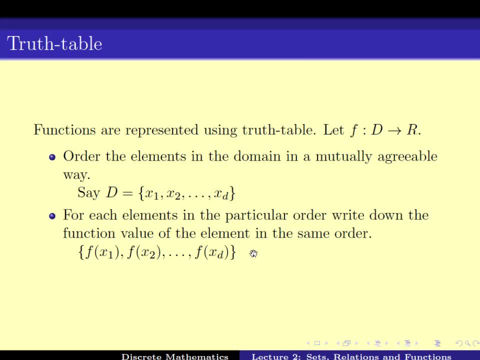 in the ordering that I give you is a mapping of X3 to the range. Similarly, maybe, the ordering of the domain set. Similarly, maybe the tenth element here is a mapping of X10.. This particular description of the F, by giving you the f of X in a pre-determined order, is 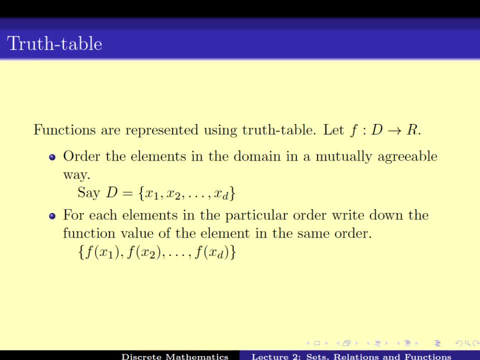 called the truth table. Thus, the size of the truth table is always equal to the size of the domain. Okay, Thank you. Now in this course there will be one particular type of functions we will be looking at bit more carefully. 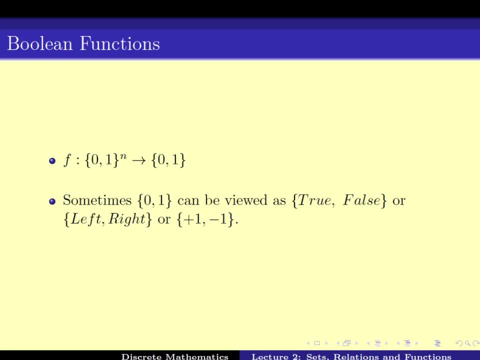 These are called the Boolean functions. So Boolean functions are functions that take values or the domain set is 0, 1 to the n, the n-dimensional hypercube, and it outputs 0, 1.. This 0, 1 can be viewed in different ways. 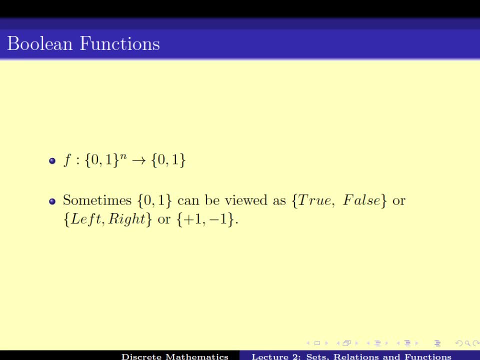 You can think of it as 0 representing true, 1 representing false, or 0 representing left, 1 representing right, and so on and so forth. Depending on our need and the context of the problem, we will interpret the 0 and 1 differently. 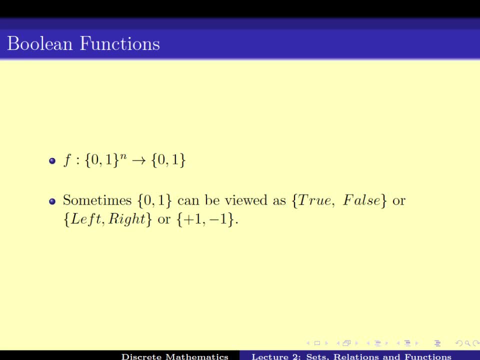 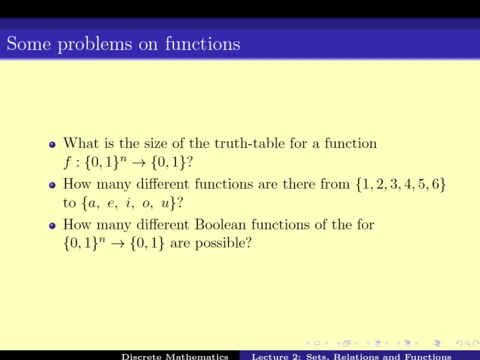 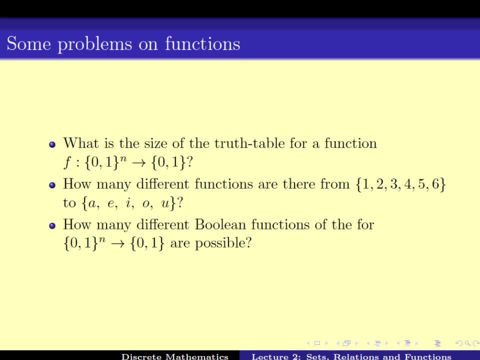 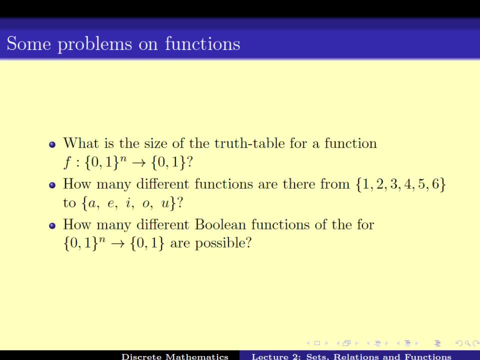